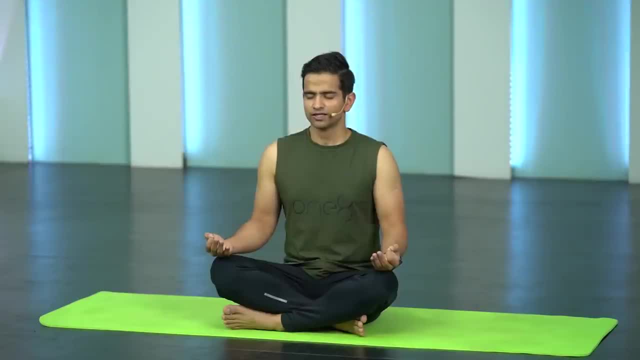 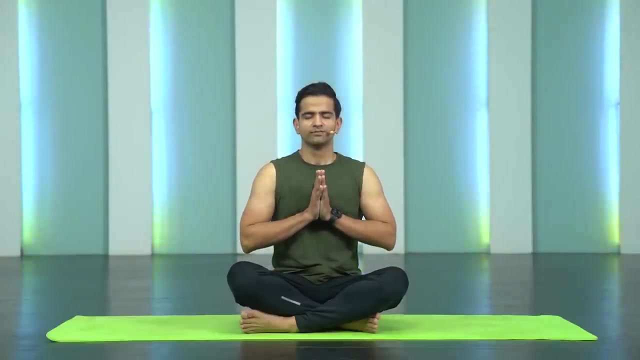 Keep observing the energy of this affirmation all throughout your body. Let this affirmation become one with you. Bring your palms together in namaste. We'll invoke the energy with omkar: Inhale Aum, Aum, Aum, Aum. 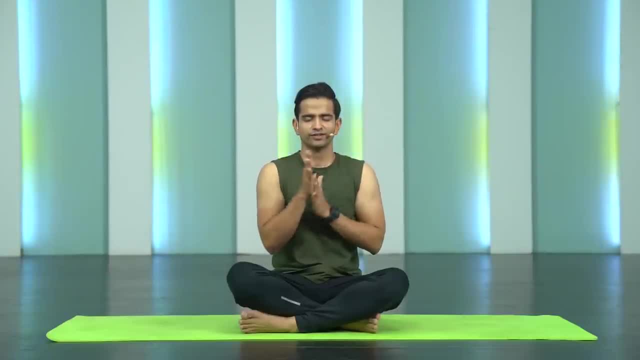 Now, very slowly, start to rub your palms, creating good amount of energies in your palms, Bringing your palms to your face. Energize yourself and look at your palms with a beautiful smile and a few blinks, All right, So let's get started now. 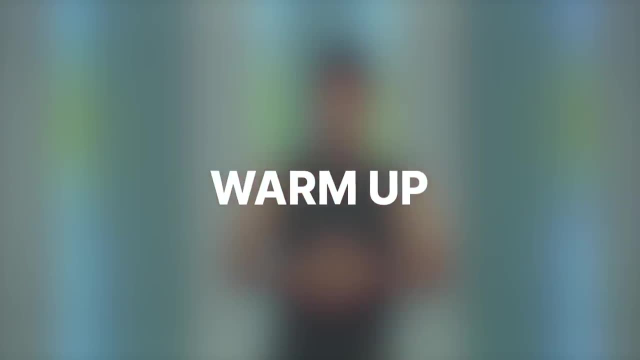 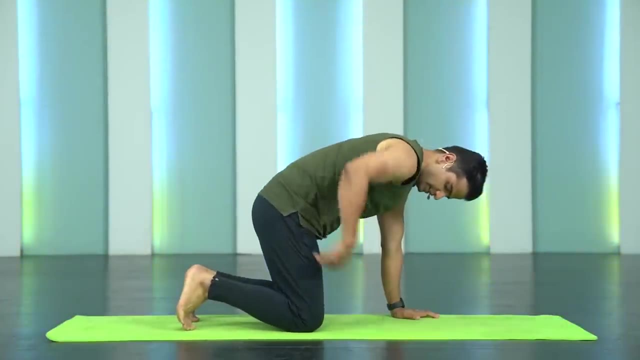 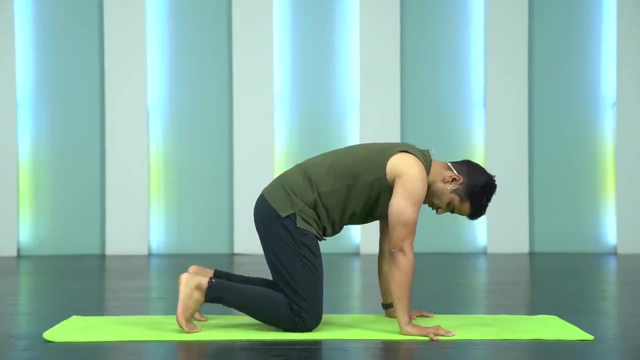 Let's come to the table top position for the warm up. You will take your wrist exactly below the shoulders. Your knees will be exactly in line with your pelvis. Now just look at me what exactly we will do From here. you will turn your toes in, keeping your legs slightly wider. 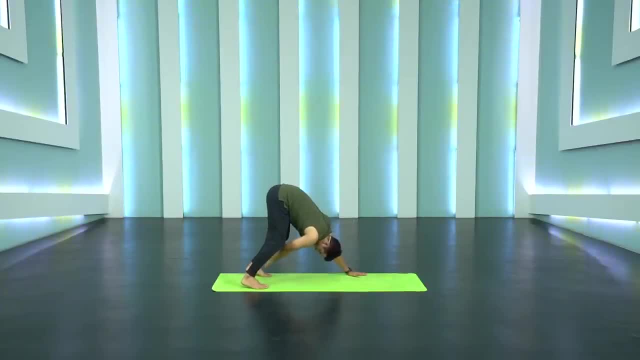 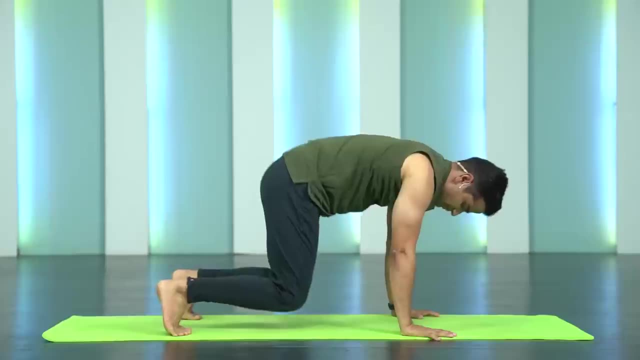 You will push back like this: taking your right palm to the left ankle, Bringing it forward, Left to the right, Bringing it forward and then again bringing your knee down. So that's how we will keep moving from table top to the downward facing dog twist. 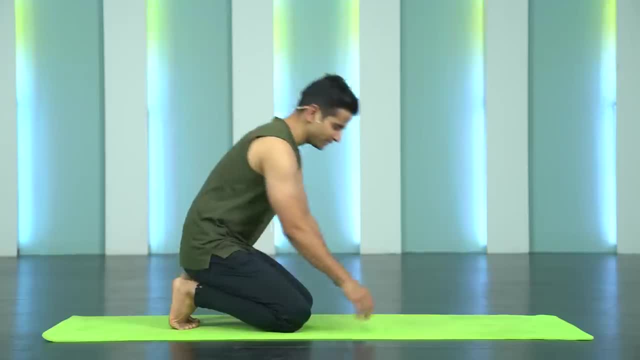 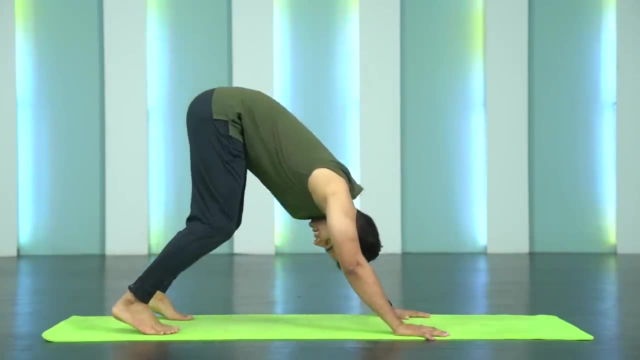 Now let's go ahead for total five rounds, with the same Coming here Turning your toes in legs wider. This is important. Now push back with the knees gently bent. Take your right palm to the left ankle. Right hand goes forward. 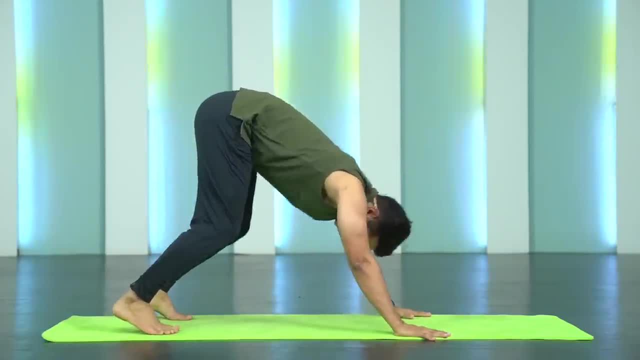 Left to the right, Left goes forward and down. Let us slow it down with the breath. So inhale here, Exhale. Pushing back, Taking your right palm to the left ankle Right goes forward Again, inhale, Exhale. 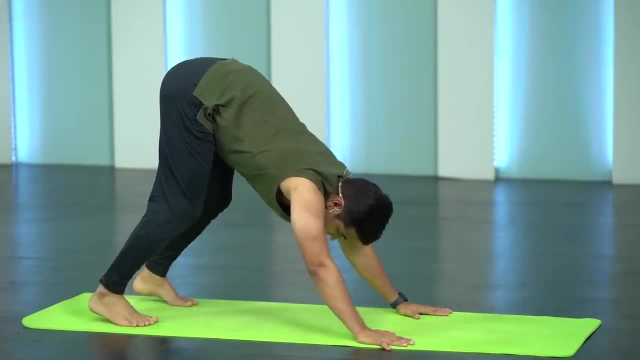 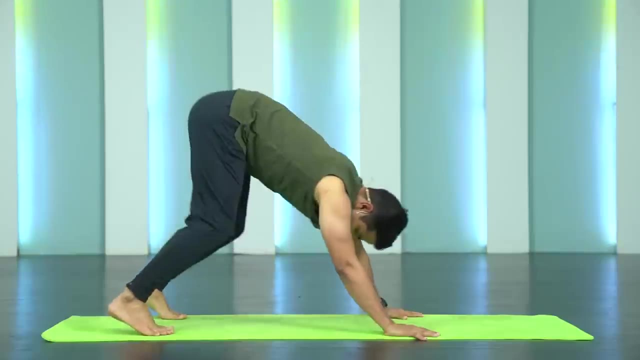 Take your left palm to the right Again inhale here Exhale. Take your knees down. Let's go for the third round Again inhale, Exhale. Right goes to the left, Forward Exhale. Left goes to the right. 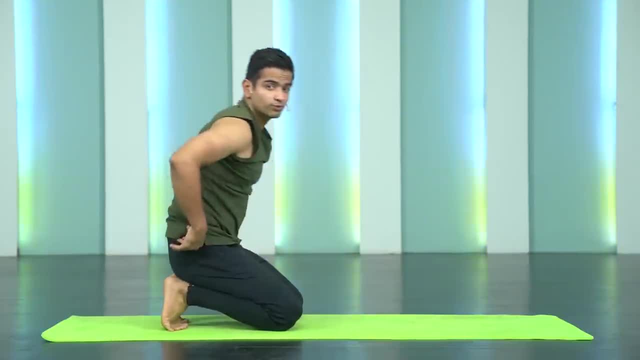 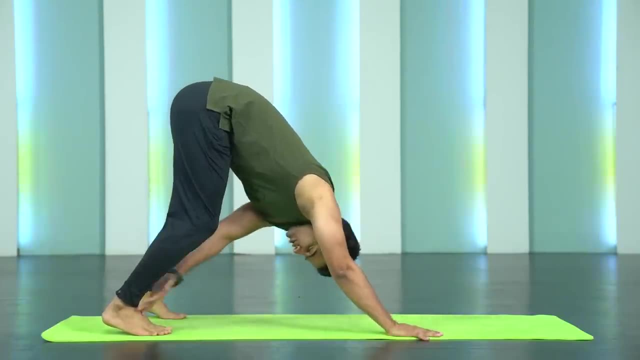 Forward And down. Let's go for two more rounds. Take a deep breath, Inhale, Exhale. Right goes to the left Forward, Left goes to the right Forward, Taking your knees down One last time. 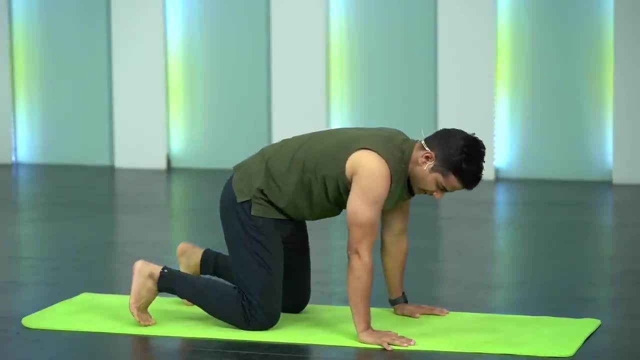 Pushing back: Right goes to the left, Left goes to the right, And then slowly take your knees down. Just relax, Take a deep breath, Inhale here, Exhale it out, completely, Inhale, Exhale. 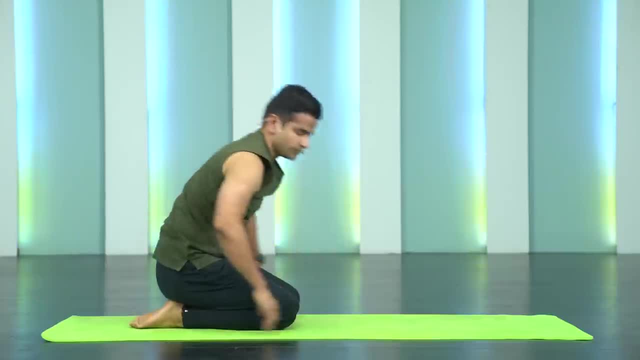 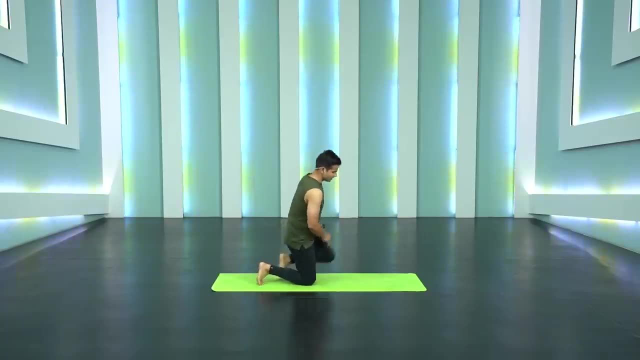 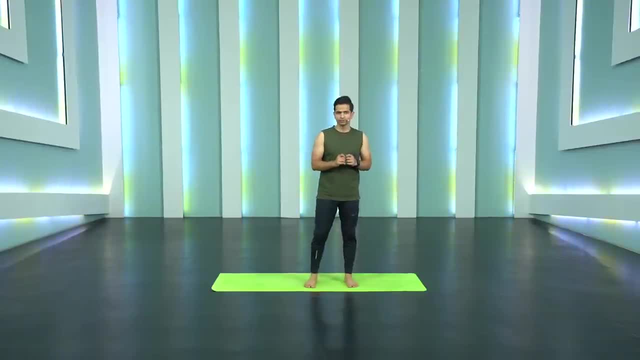 Exhale Inhale Exhale Exhale Inhale, Exhale Exhale Exhale Inhale, Exhale Exhale Exhale Inhale. 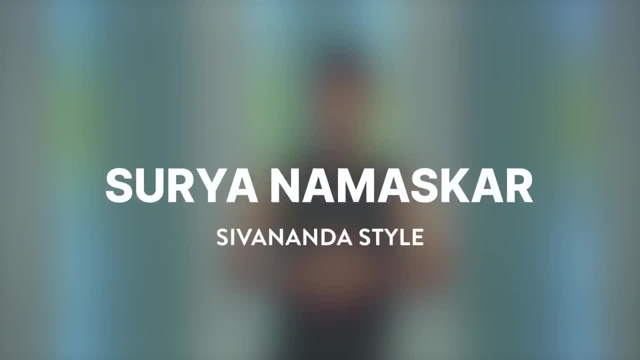 Exhale, Exhale, Inhale, Exhale, Inhale, Exhale. And then let's lift it up and then gently coming up. So we have learnt Surya Namaskar in the last session. 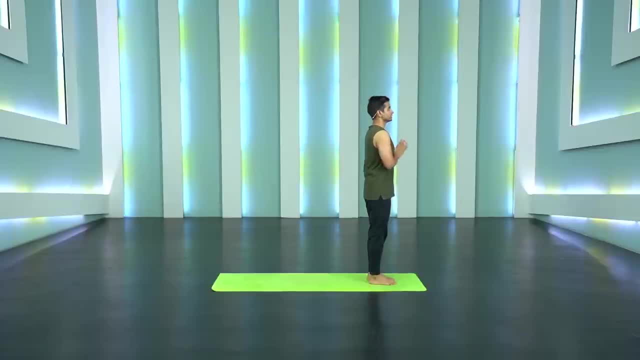 We're going to be doing the same Surya Namaskar, but today we will take it an notch higher by practicing total 3 cycles. Let us do it together: Inhale, raising your arms, bending your knees forward and then looking up. Nice. With exhale, keep your knees bent, only leaning forward down. With inhale, take your right leg back as far as possible, taking your right knee down, and look forward. 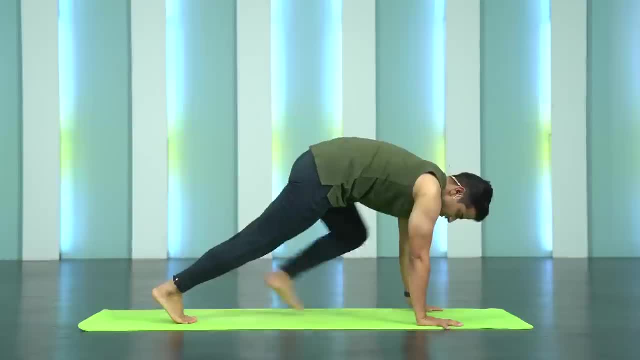 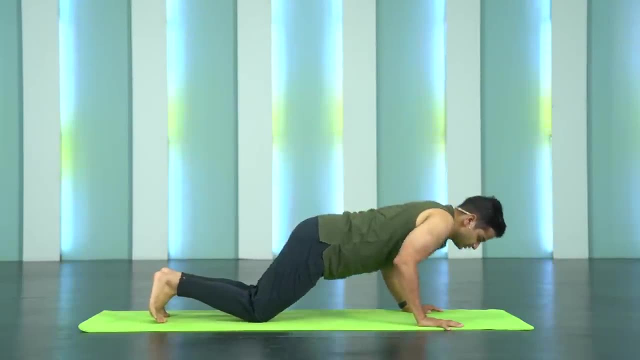 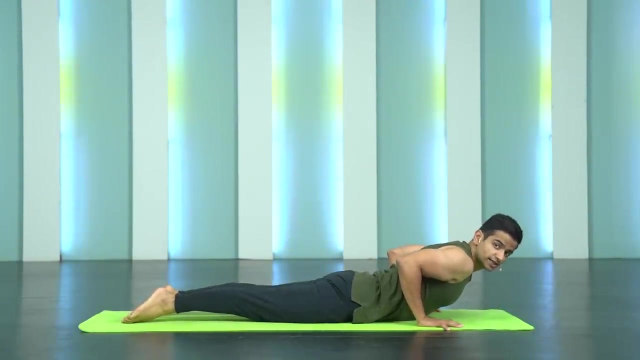 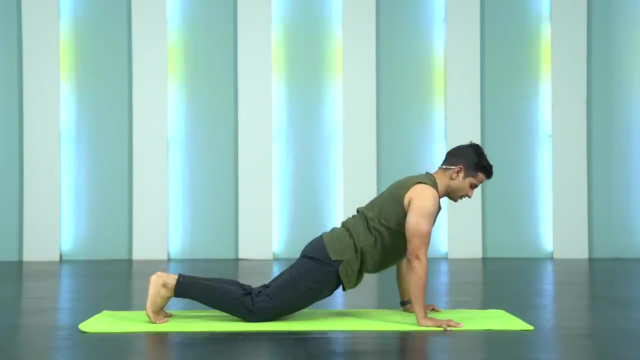 Ashtanga Namaskara. Let us take the left leg back, Inhale here again. Exhale taking your knees down, Take the chest down, chin down Ashtanga Namaskara And then inhale coming up to Bhujangasana. here, Make sure your legs are together, Tighten your glutes, Turn the toes Slowly, come back, First your upper body, then lower body And then we push back nicely into the mount. 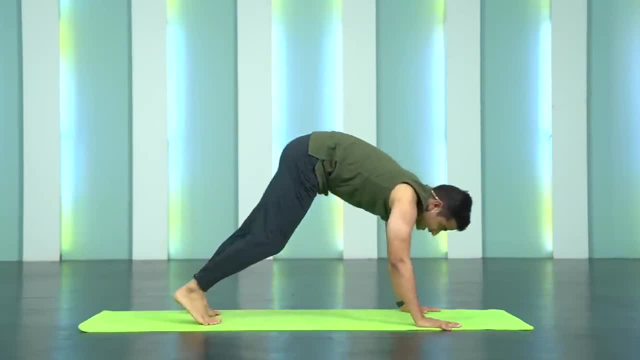 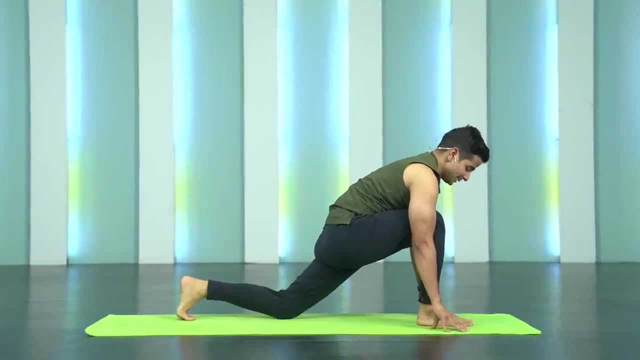 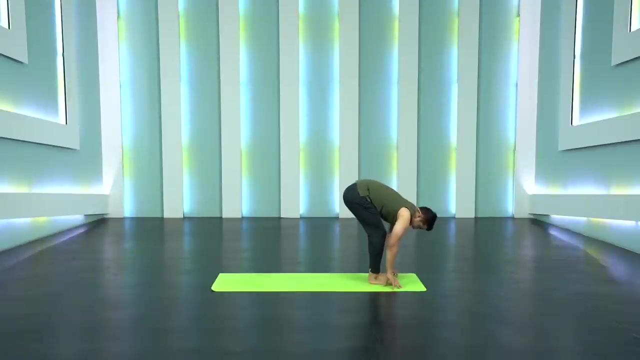 In position. From here, let us take our right leg forward. We keep the left knee down Again, inhale Ashtanga Namaskara. Exhale, your left leg will go forward, Both the knees bent, Holding it here. Padahastasana. Inhale, lifting your hands up higher, Gently bending back, pushing your hip forward, And then exhale Pranamasana. That was first half. Only 12 steps we have done. 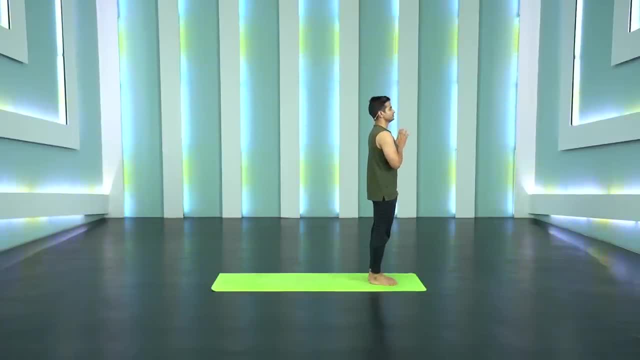 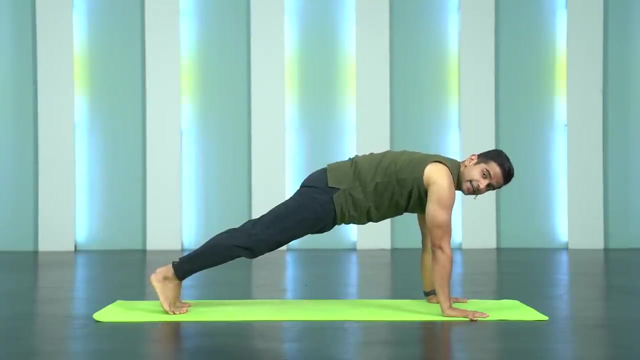 Let us do Another 12 from the left side Palms together: Inhale Hastuttanasana, Gently bending back. Exhale, leaning forward down with the knees bent Now. inhale, left leg goes back. Take your left knee down, Toe out. if you feel like Look forward Now, turn the left toe in. Right leg goes back Again. inhale- Exhale. take your knees down, Chest down, chin down. 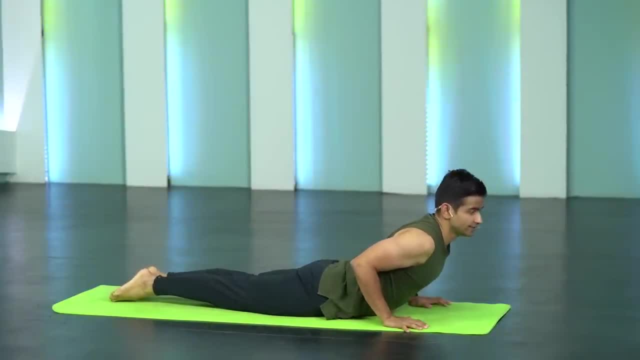 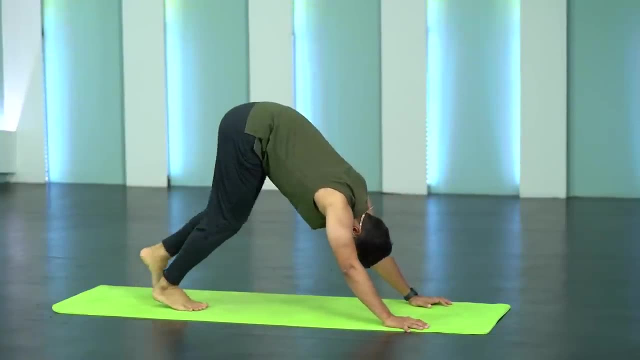 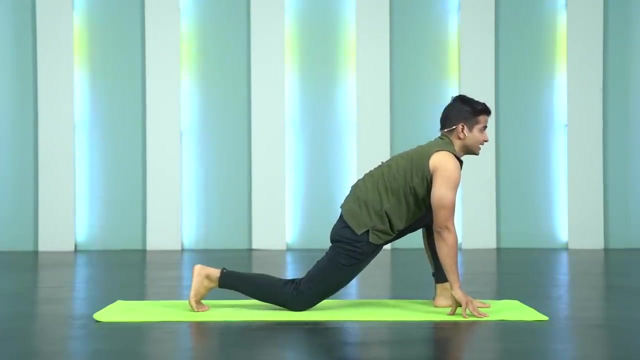 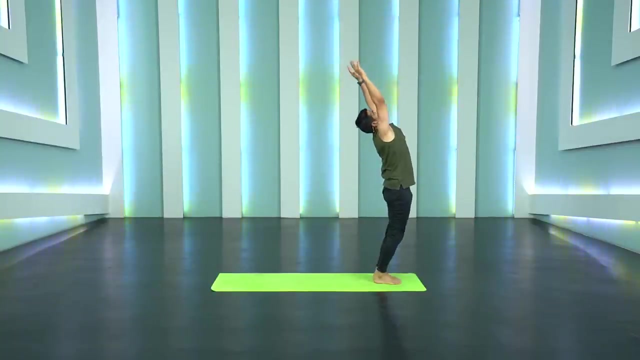 And then, legs together, completely Lift your chest in Bhujangasana Cobra pose, Turning your toes. Push back to Parvatasana Mountain pose. Let us take left foot forward, Adjusting the right here. Inhale, Exhale, right goes forward And then inhale, Raising your hands up higher, Gently bending back, Coming back to Namaskara. 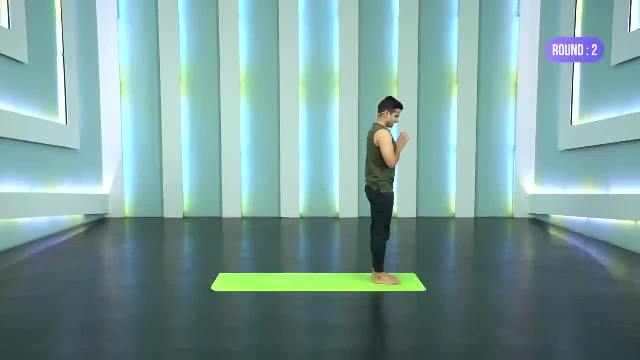 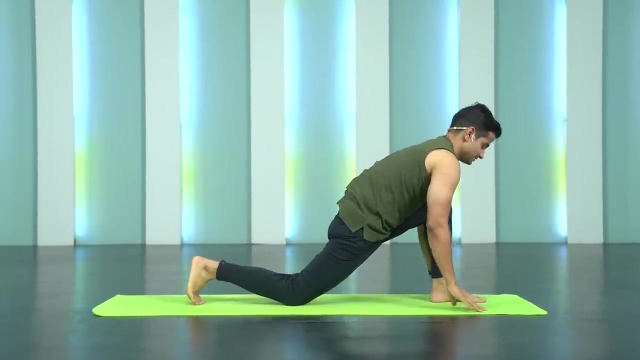 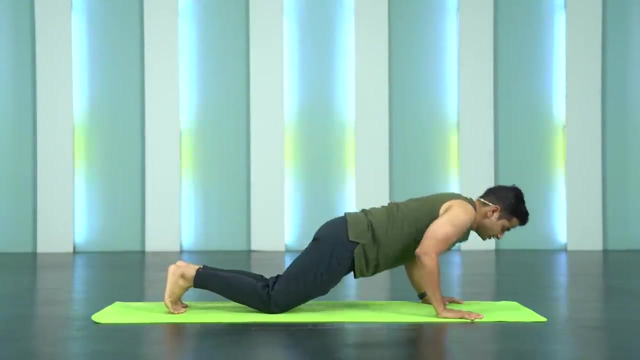 We are done with one round. Two more Again. Pranamasana: Inhale gently bending back. Exhale leaning forward down Knees. bent Inhale, right leg goes back And you look forward Slowly exhale. take your left leg back Again. inhale And then exhale, taking your knees down Chest and the chin down. Your hip will be slightly higher. Then inhale Coming up to Bhujangasana. 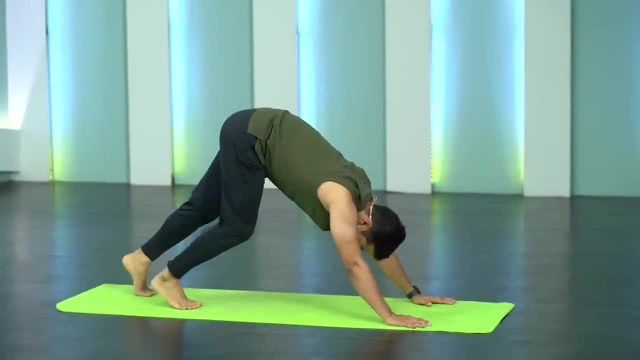 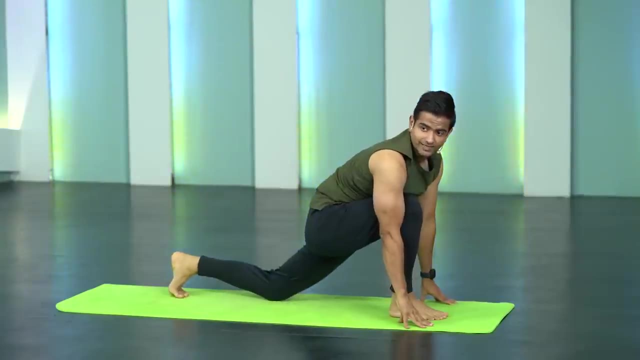 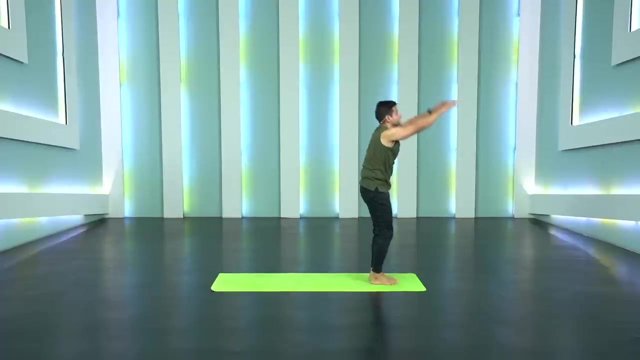 Turn your toes in, Move back to our mountain position. Slowly we'll take right leg forward. Left knee will be down. Look forward. Inhale With exhale. left leg goes forward And then inhale Gently bending back, Exhale Namaskara. Another half Again inhale Gently bending back, Exhale down. 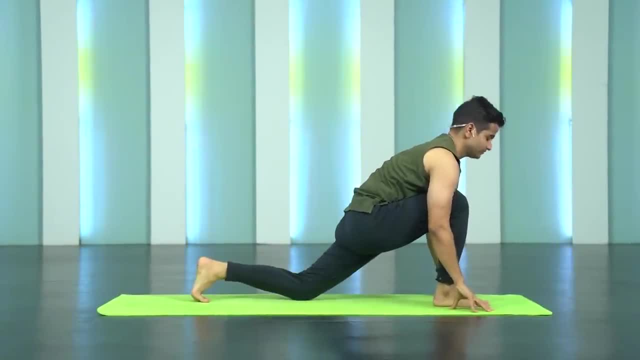 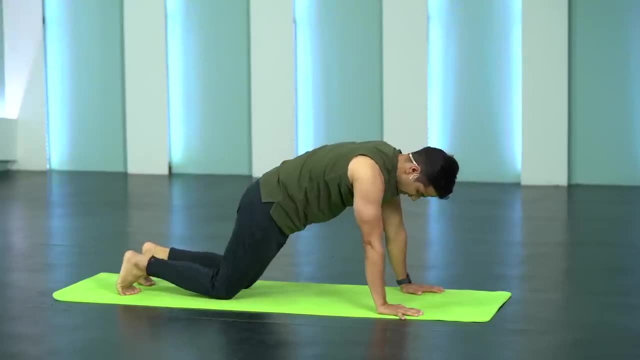 Take the left leg back, Look forward, Inhale secondo el kuosh ej and then exhale. Right leg goes back, Coming in to Dandasana or Santo Lanth, dreamed. Exhale knees, chest and chin down. 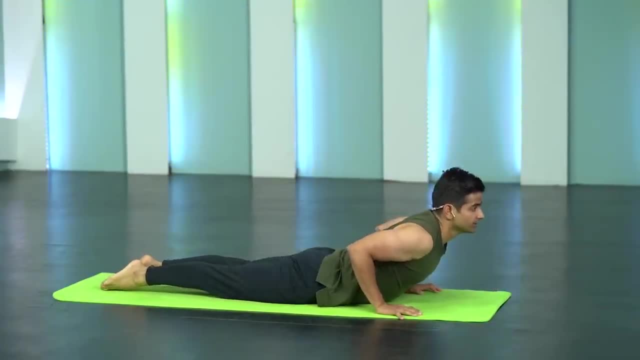 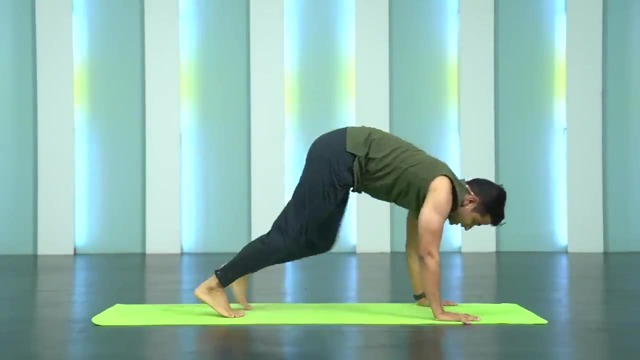 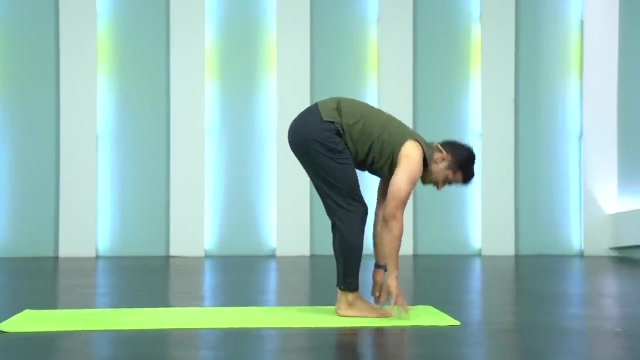 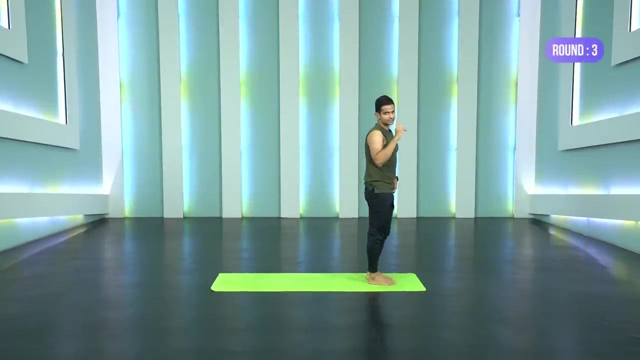 Stand on Namaskara, Inhale Bhujangasana, Turn your toes in, Push back Mountain. Let us take the left leg forward, Right knee down, Yea. Exhale right leg forward and then inhale gently, bending back, exhaling pranamasana. wonderful, one last cycle to go. 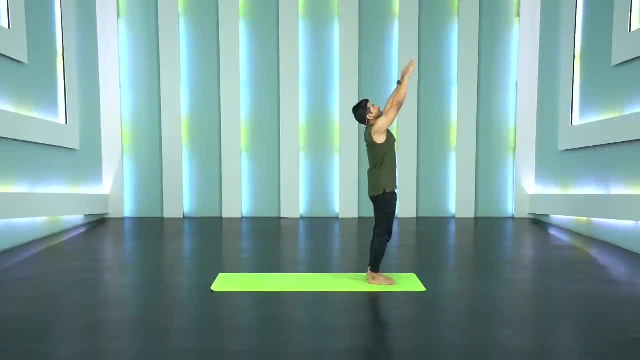 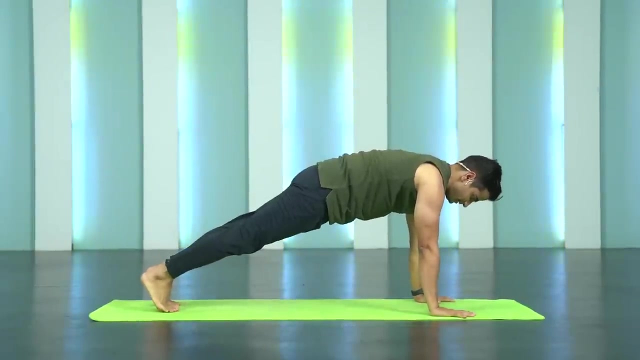 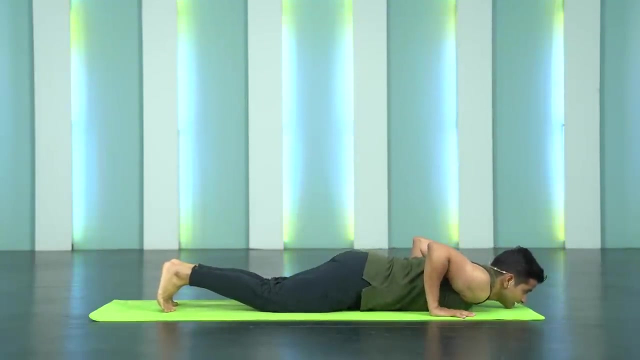 all right together, palms together in namaste inhale gently bend back. exhale leaning forward down. take the right leg back, right knee down and look forward. exhale- left leg goes back inhale here. exhale knees down, chest and the chin down. now legs together coming up to 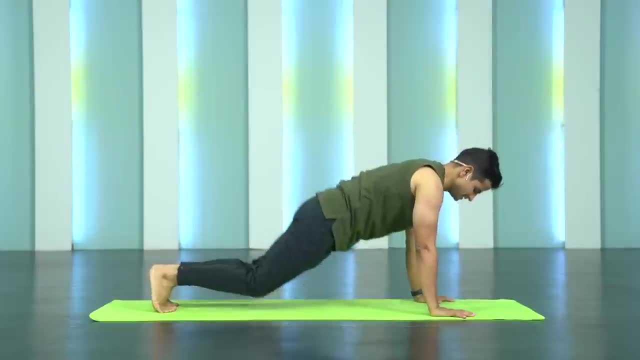 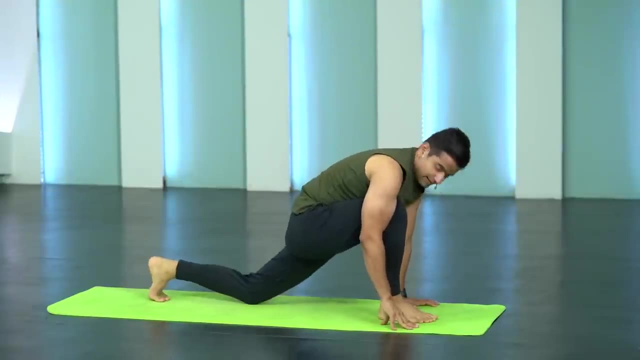 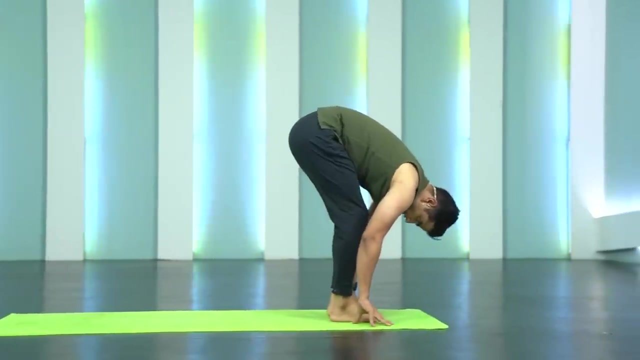 bhujangasana. turn your toes in. exhale. slowly push back to mountain. right leg goes forward, your left knee will come down. push the hip forward, look forward, inhale- exhale. left leg forward: inhale. gently bend back. 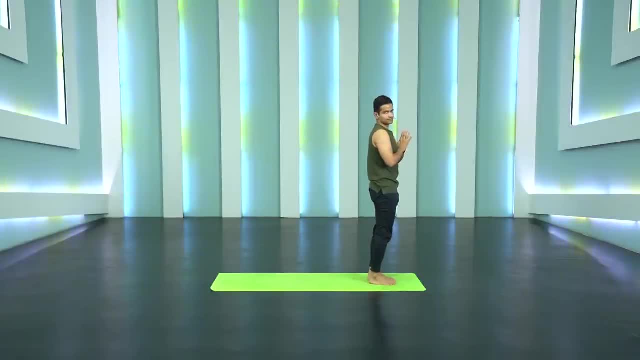 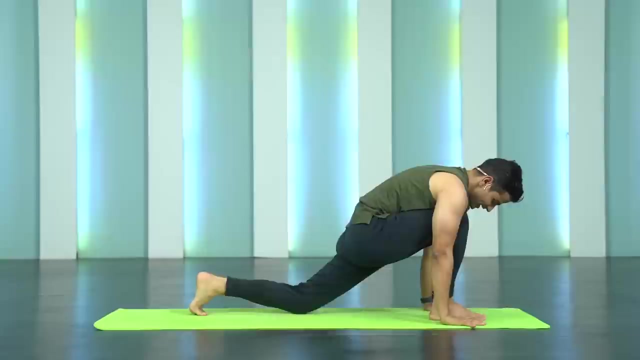 bending back, exhaling- pranamasana. last half again pranamasana. inhale gently bending back. exhale, leaning forward down your left leg goes back. look forward. inhale, exhale, right goes. 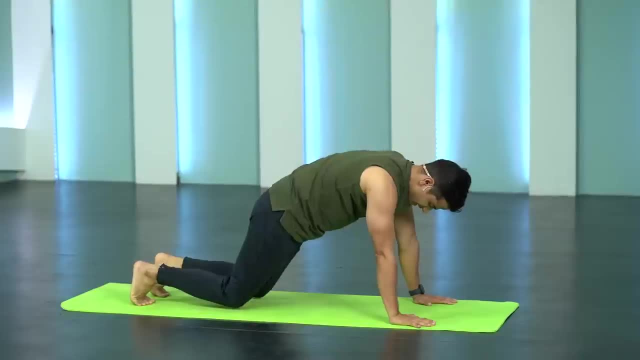 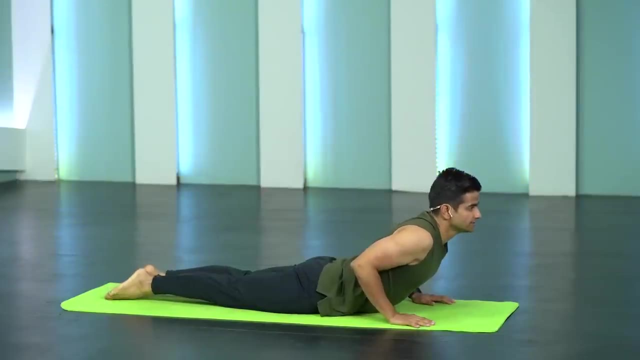 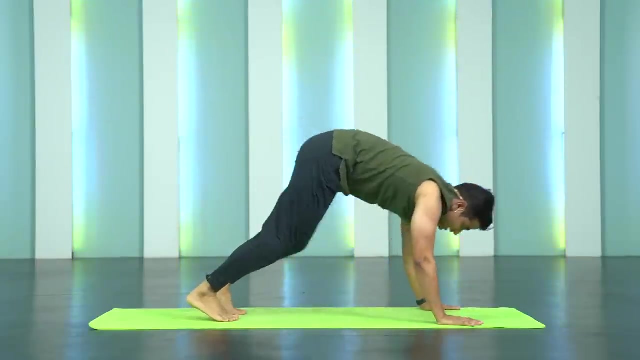 back inhale again. exhale knees down chest and chin down, then slowly cobra bhujangasana exhale. move back to parvatasana mountain. gently take your left leg forward, looking forward. 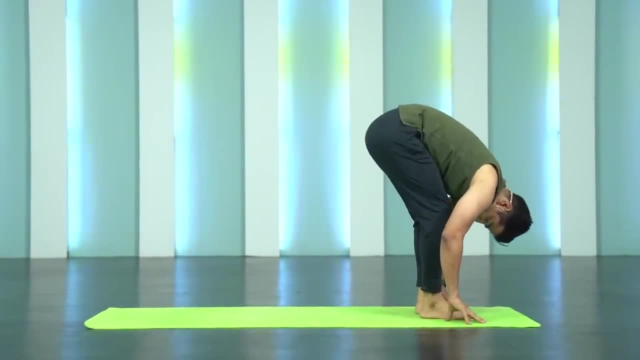 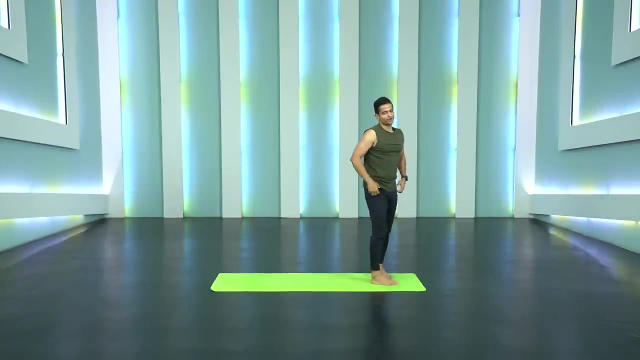 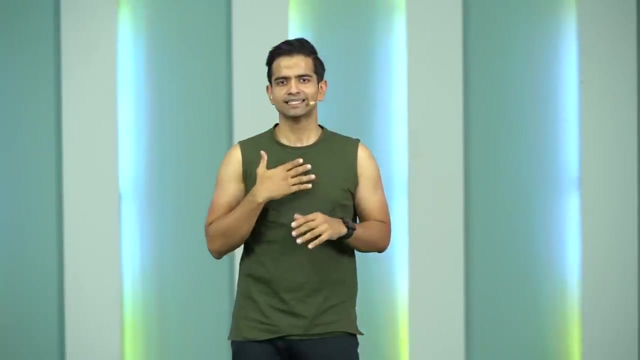 inhale, exhale right forward and then inhale bending back. exhale pranamasana. all right, so we are done with total three rounds of shivananda style. surya namaskar, I know heart rate. 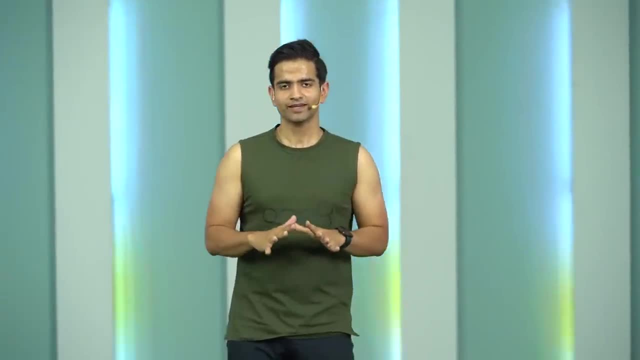 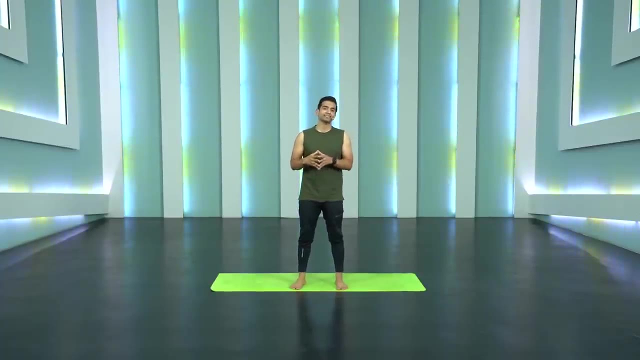 breath rate. both will be higher right now, so you keep calming down. meanwhile, I will tell you the idea that I was about to share. now, we mostly forget about our healthy habits because we don't really keep a trigger for it. 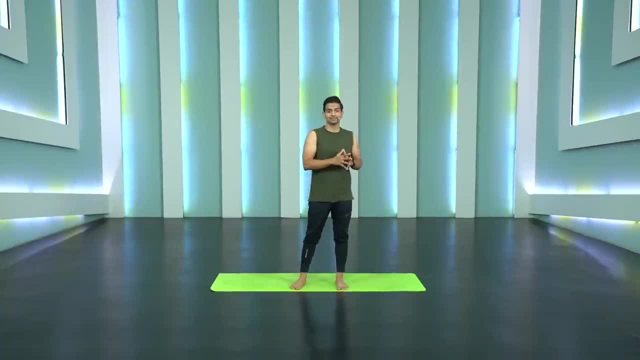 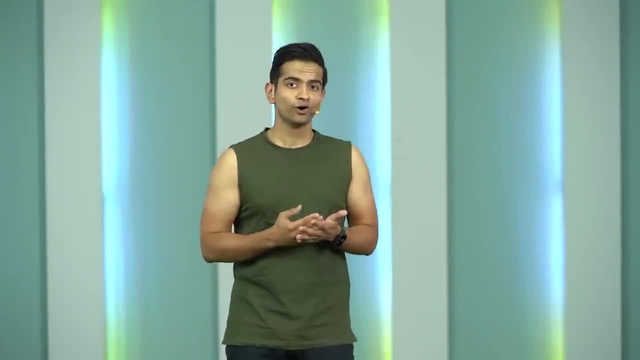 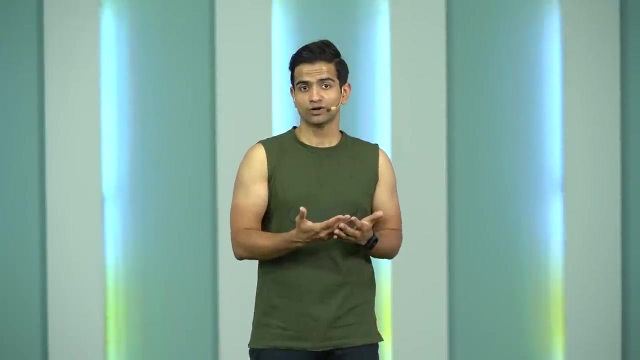 everything that we do all throughout the day goes with a trigger for healthy habits. we hardly have it right, so all we need to do is to just write your healthy habit on your paper. keep it in places that you maybe sit and work mostly, that you maybe see all throughout the day. 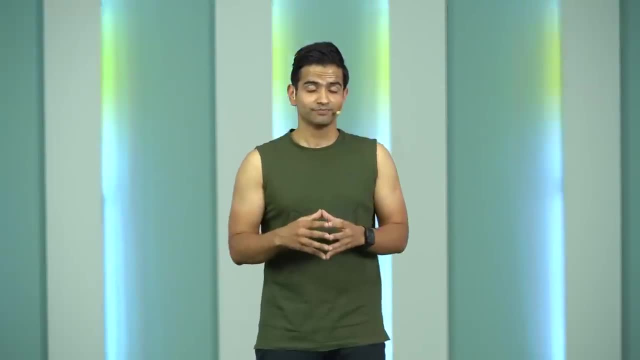 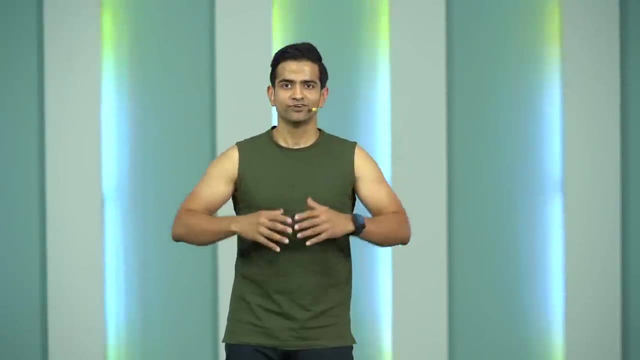 it could be a cupboard, it could be a fridge. now, what will happen when you keep that? whenever you are sitting there, whenever you are walking to those places, every time it will give you the reminder of that habit. for example, hydration. 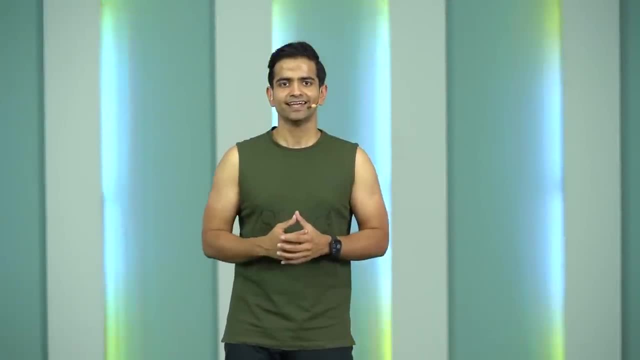 now, if you want to drink water, just write that on that and every time you see that you will get reminded of drinking water and you will drink water. the chances of you doing this will be a lot higher than you are doing it without that. 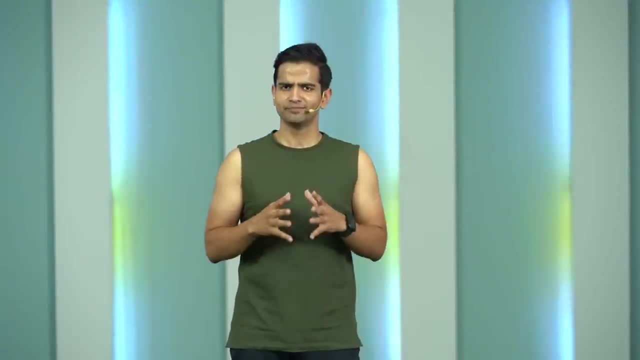 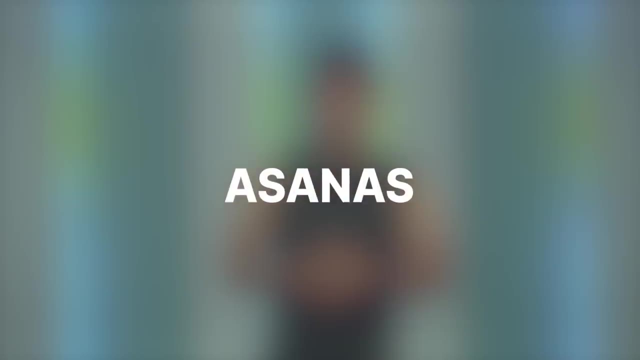 so that's the idea that I wanted to share. make sure you follow this and let me know how it works for you. now let's go ahead for asana. as your breath rate, heart rate, is sorted already, we'll start with our first asana, which is going to be standing. 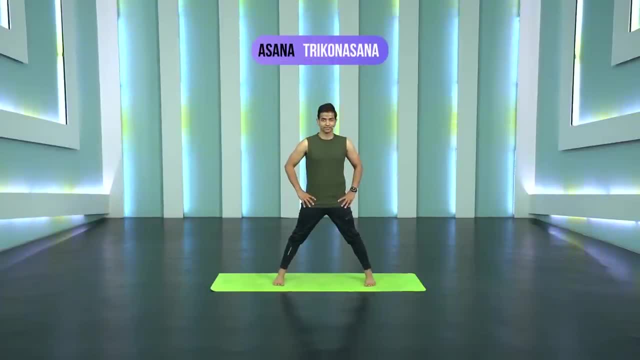 so open your legs wide for this asana trikonasana, and turn your right toe to the right side. alright, left toe will be slightly diagonal, perfect. now gently take your right palm to the right shin. it is just below your knee. 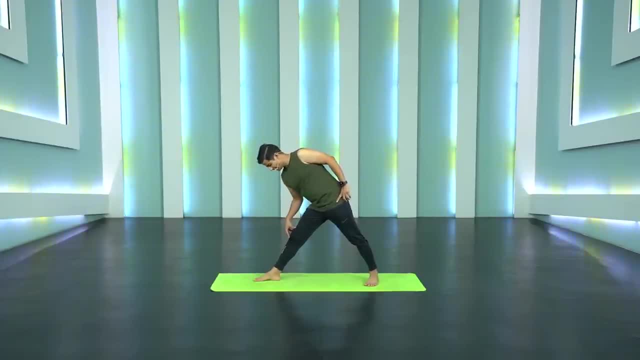 but do not push your knee too much behind. you can have it slightly your right knee bent. keep your right palm here and then pull the left shoulder behind with me. come until here and then slowly raise your left hand up high. that's it. 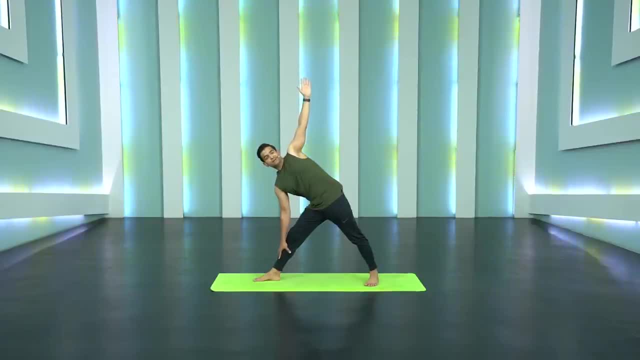 we are already in the asana, so let's just hold this asana for the next five breaths, holding it here: one breathe. two: inhale and exhale. three: make sure the knee is slightly bent. four breathe: 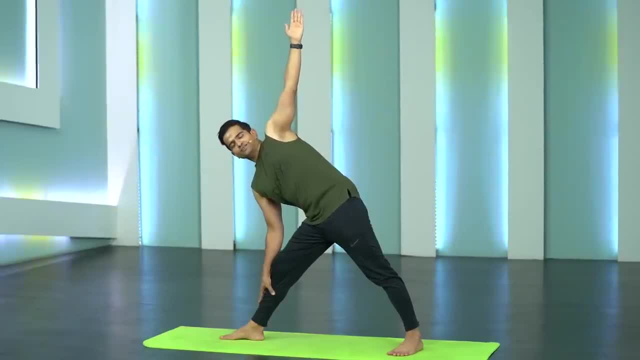 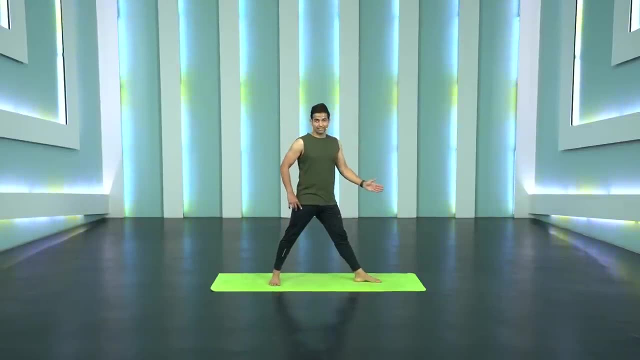 and five. wonderful. very slowly, we'll come back. now turn your right toe to the front and then take your left toe to the left side. just bend your left knee micro. okay, now take a deep breath, inhale. your torso is towards me, left palm below your left knee. 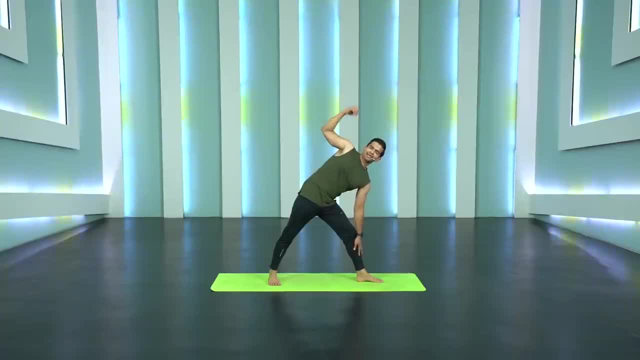 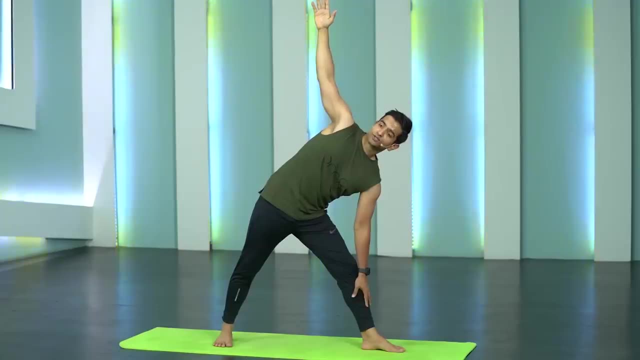 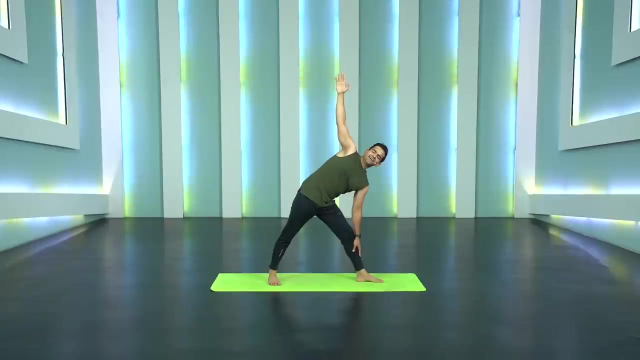 pull the right shoulder behind as much as the body allow and then take your right hand up high. that's it, holding it here. one breathe in and breathe out. one, two, three- almost there- four and five, very slowly coming back. 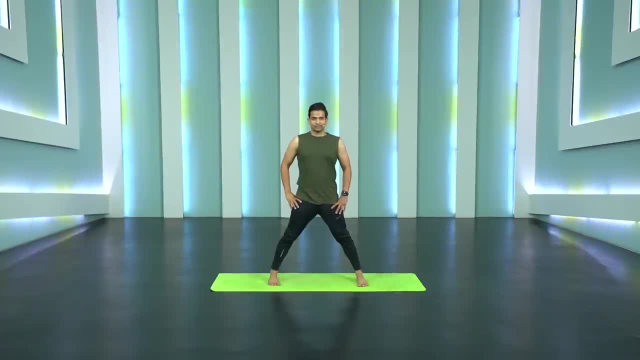 take a deep breath, inhale and exhale it out. now, gently bring your both the legs together. we will sit down and going ahead for our next asana. the next asana is Janu Sirshasana. what is Janu? Janu is your knee. 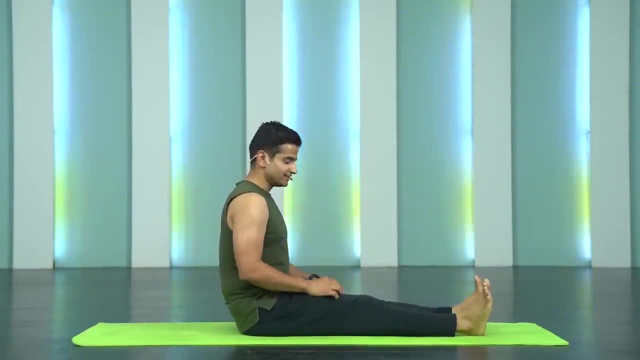 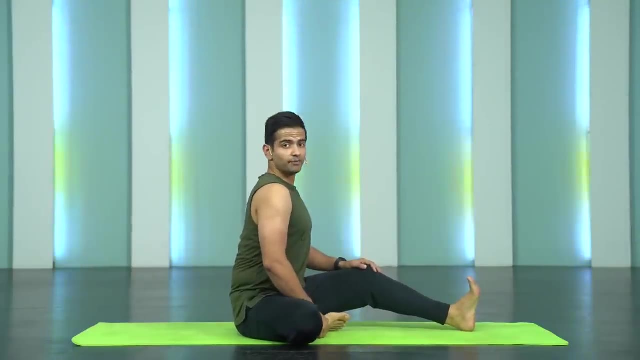 that is why the name is Janu Sirshasana. so quickly, look at the demonstration. you will take your right leg behind and you will have your left knee slightly up and you will keep your back up higher and then, slowly, you will try to lean forward. 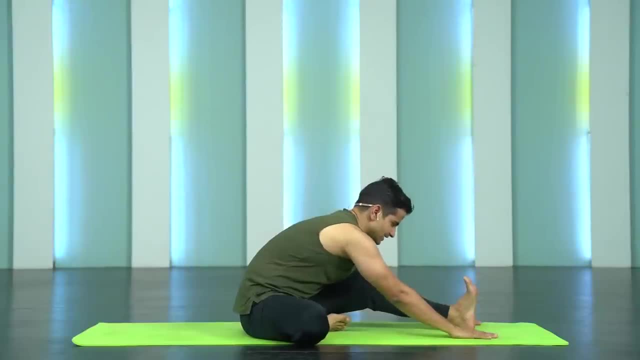 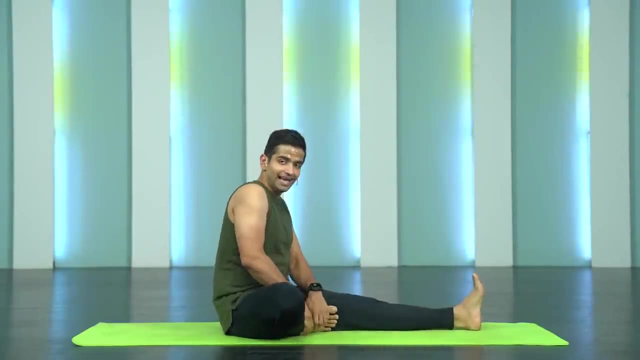 either taking your palms to the side or you will take the hands slightly forward, and that's it. this is what we will be doing right now. so let's get started. take your right leg back and keep your back straightened. let us lift the left knee slightly higher. 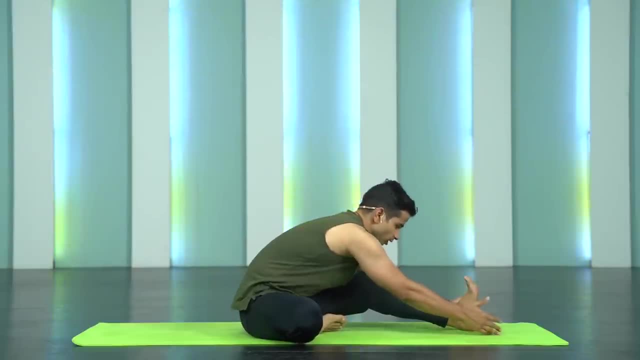 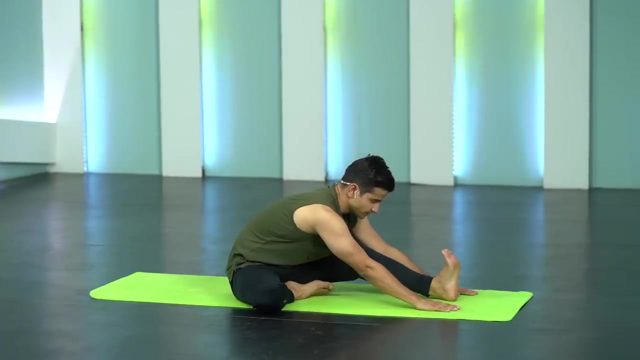 pull the left one towards you, and either you will go forward or slightly to the side, whichever works best right now. so let's take the hands forward and stay there. one, breathing in and breathing out. hold it here: two: breathe in and out. three, four breathe. 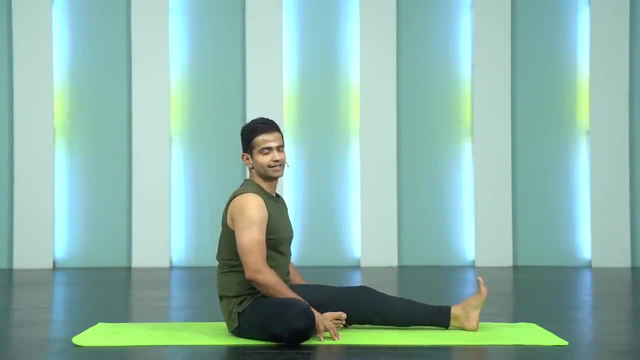 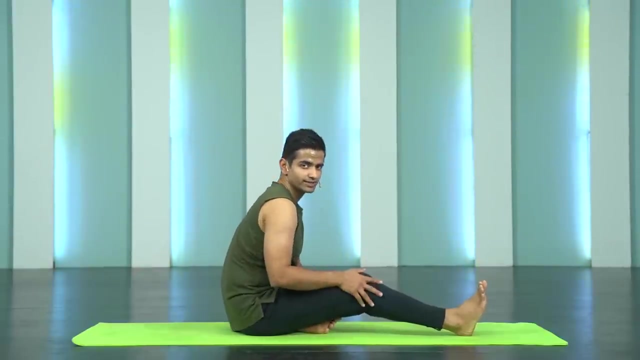 and five, very slowly coming back, straighten your right leg, we change, the side left leg goes back alright, lifting the right knee slightly, and then we lean forward. but what's happening? while we are doing this, you are getting a lot of stretches from your hamstrings. 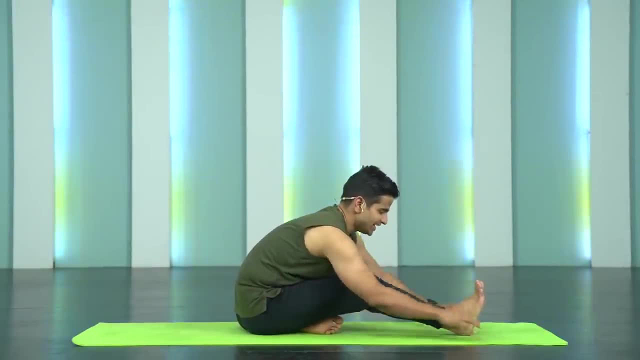 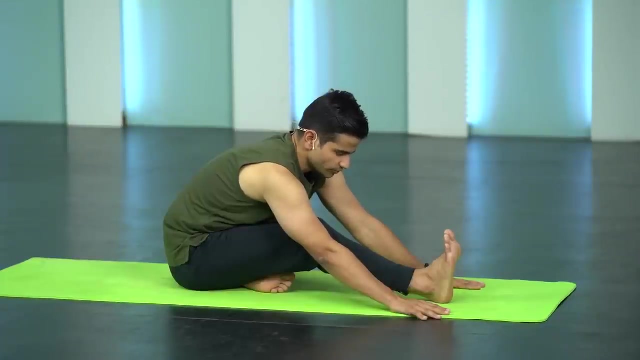 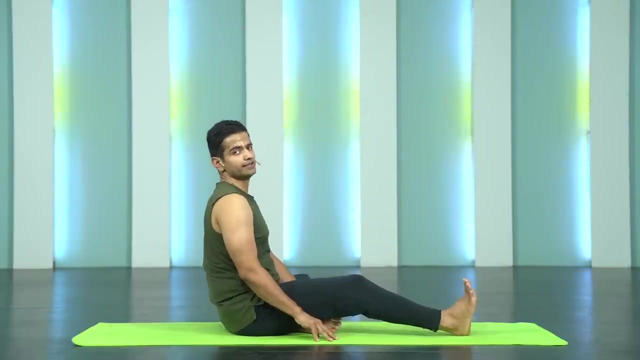 for that reason we are doing this: exhale, leaning forward, down and then stretch your hands as much as the body allow. one: pull the toe towards you. two: breathe in, breathe out. three, hold four and five. very slowly. come back up, inhale and relax. take a deep breath. 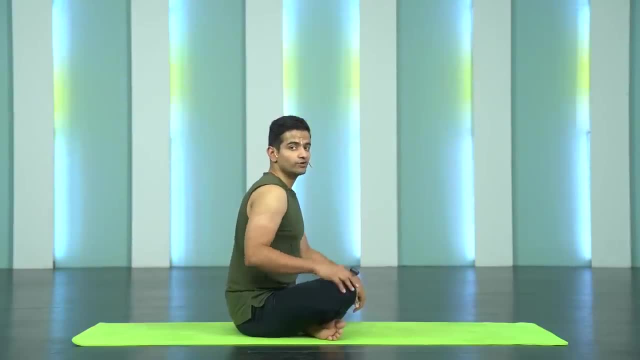 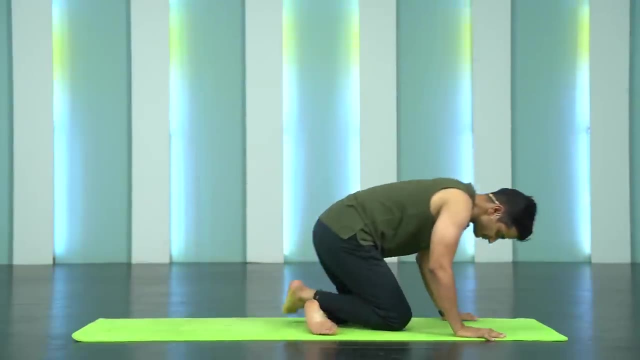 inhale here, exhale it out. let's go ahead for our next asana, which will be a prone position, meaning we will be lying down on the abdomen. so let's lie down. we will first lie down and then you can look at the demonstration. 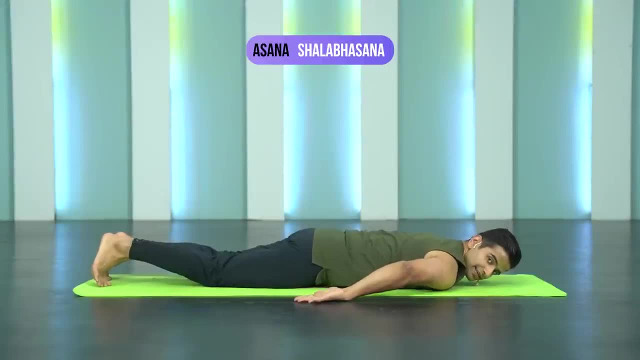 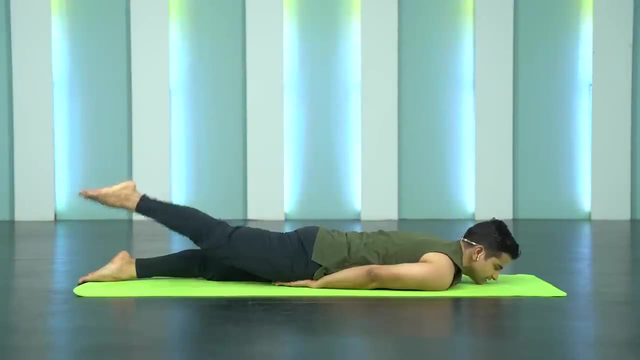 so you will take your palms below your thighs. your palms will be like this: you will take it below your thighs and then, initially, you will lift only your right leg for 5 breaths, you will bring it down and then you will lift left leg. that's it. 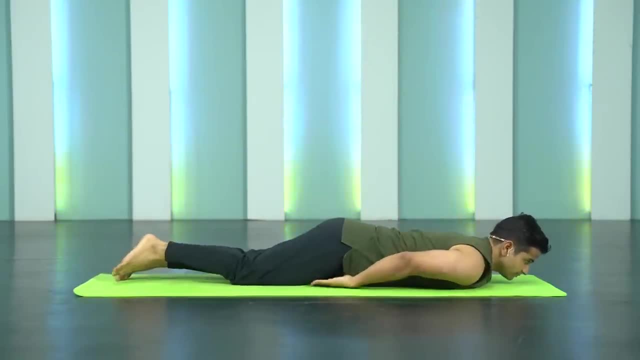 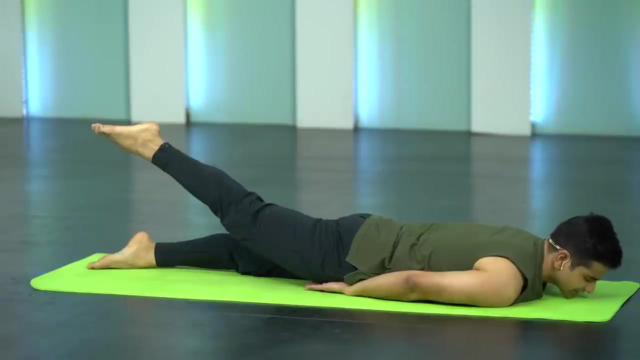 so let us do it together now. make sure both the palms are below your thighs and let us lift the right leg as high as you can. 1, breathing in and out. 2, 3. hold it there. make sure the right leg is straightened. 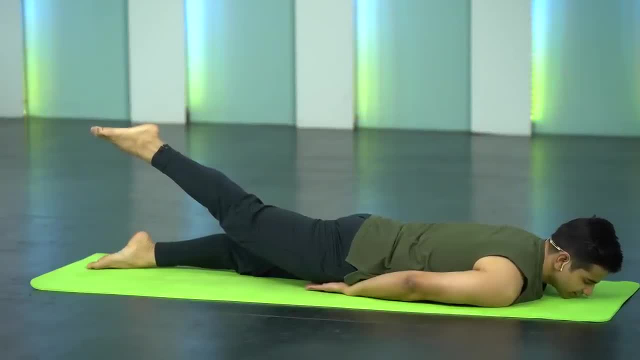 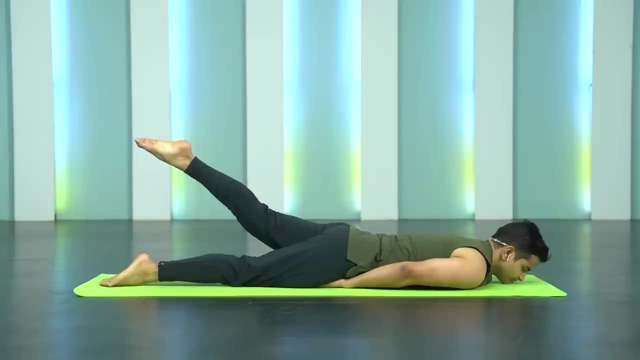 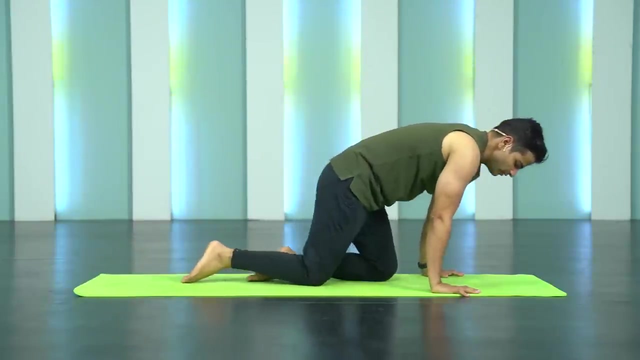 4 and 5. bring it down. change the side left, leg up higher. 1, 2, hold it there. 3, 4, 5, slowly bring it down and now take both the palms by the side. you will slowly pull yourself and then lie down on your back. 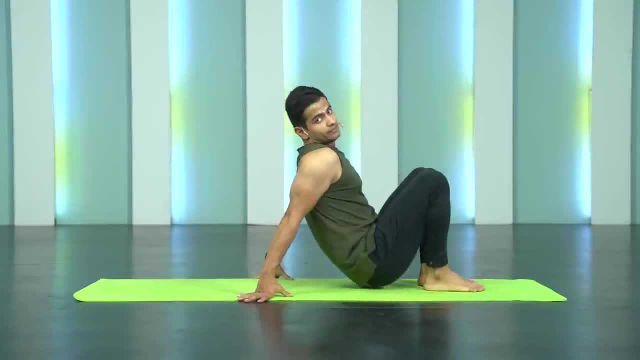 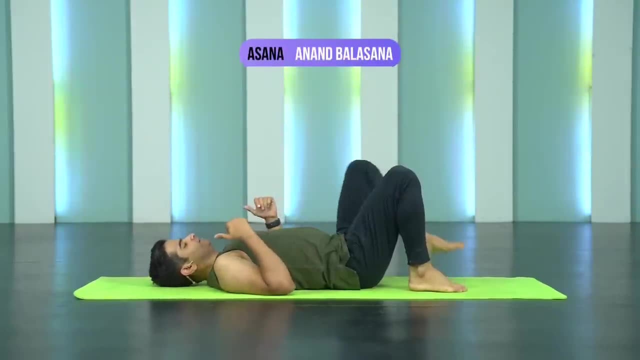 so we will now stretch the legs forward and we will lie down. you will quickly look at what we will do it and then we will do it together. so from here you will be pulling your knees towards you and then trying to grab your ankles. you can also grab your big toe. 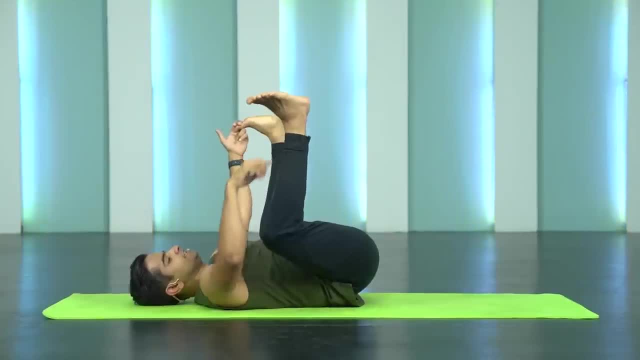 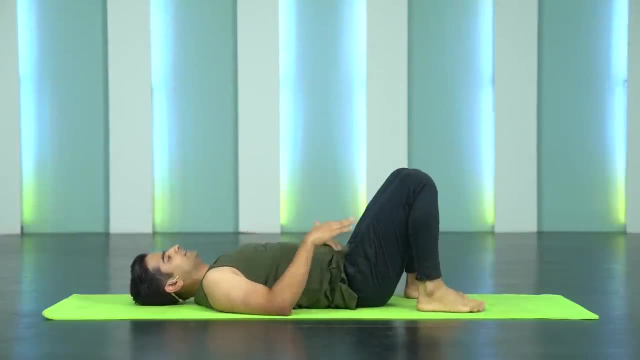 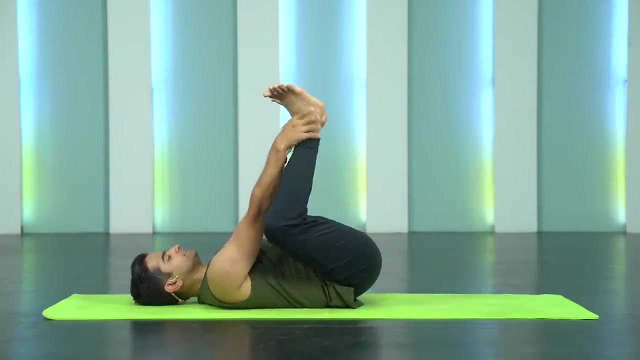 whichever works, and then trying to keep your heel almost in line with your knee. that's it. so let us do it together now. make sure you are lying down first, inhale, exhale, pull the knees, and then either you hold your ankle or go for big toe. 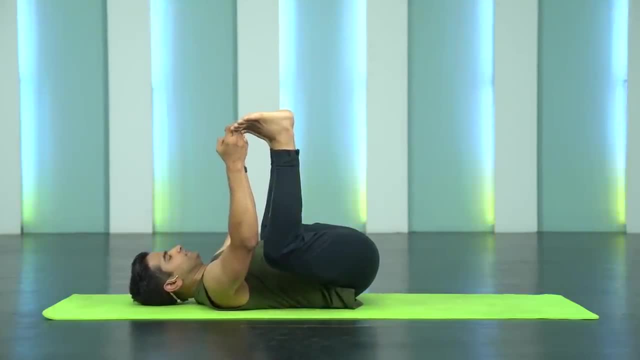 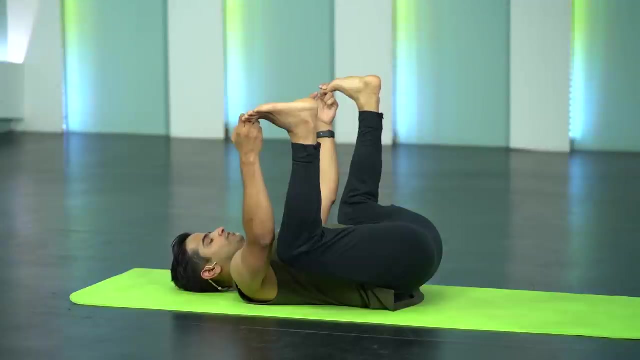 pull the heel in line with your knees and just be there. 1, inhale and exhale. 2, it's a good hip opener and you will also have the stretches from the hip region right now. 3, 4, breathing in and out. 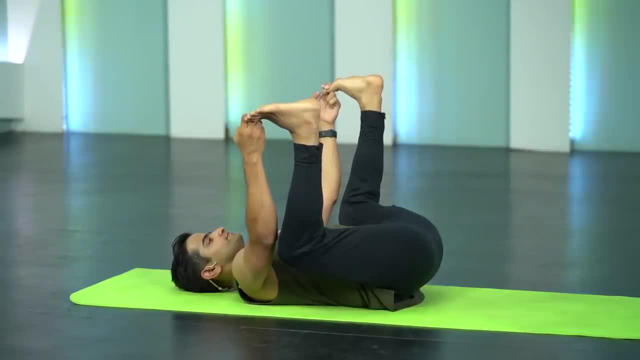 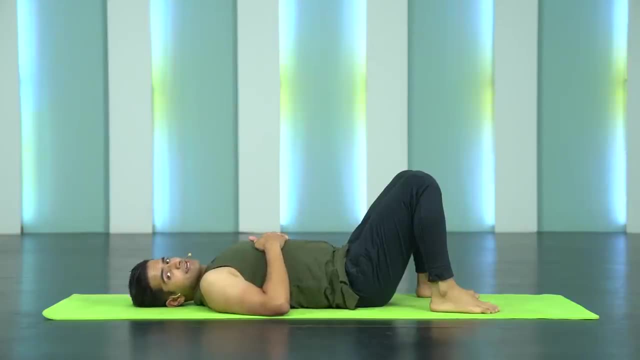 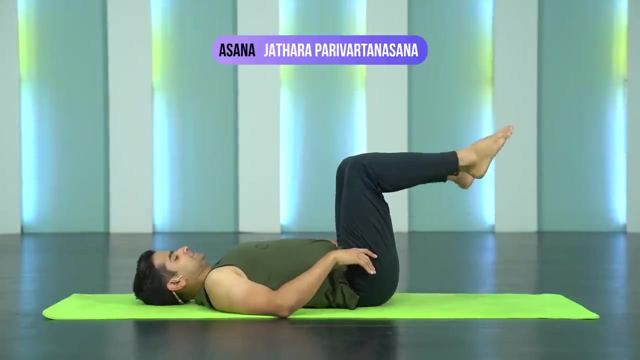 5, very slowly bringing your legs down. take a deep breath, inhale here, exhale it out completely. and now, last asana of the day. just look at me once. lift your legs like this: your knees on top of your hip, knees exactly. 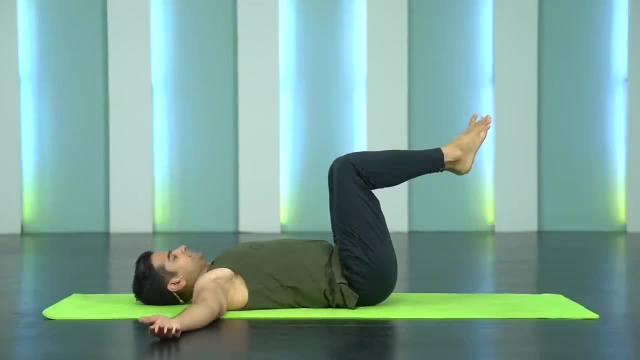 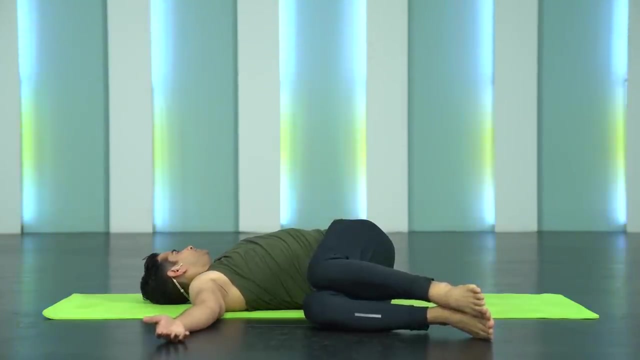 in line with your ankles, both the hands by the side. let us come to this position first. now, from here, gently, we will take the knees down to the right. so let us do it together. only we will take the knees down to the right and looking to the left side. 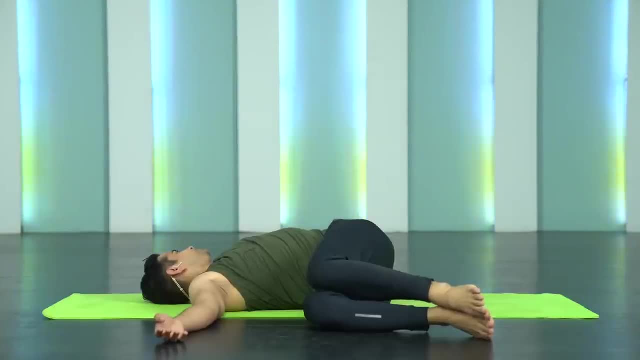 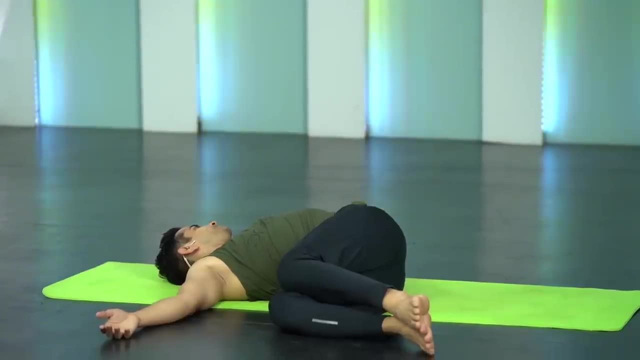 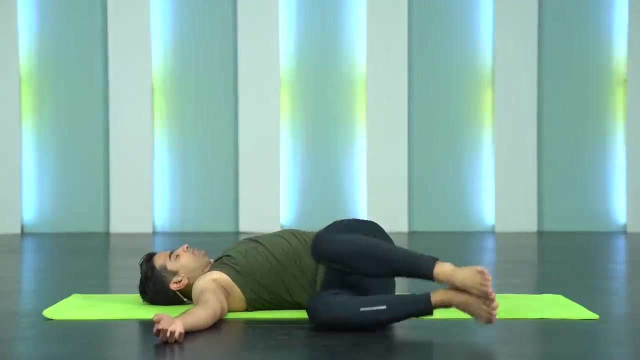 that's it, Jathara Parivartanasana, holding it here for 5. 1, 2, 3, 4, 5. slowly bring your knees back to the center. 1,, 2,, 3,, 4, 5,. slowly bring your knees back to the center. 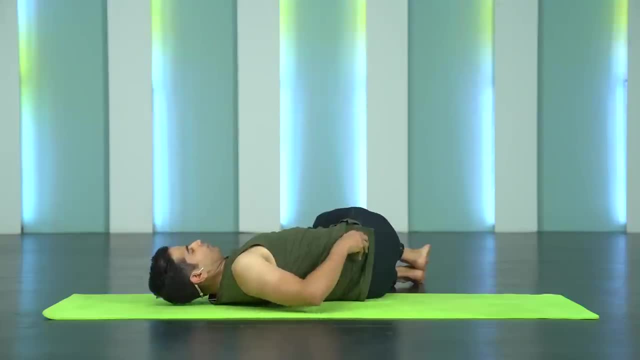 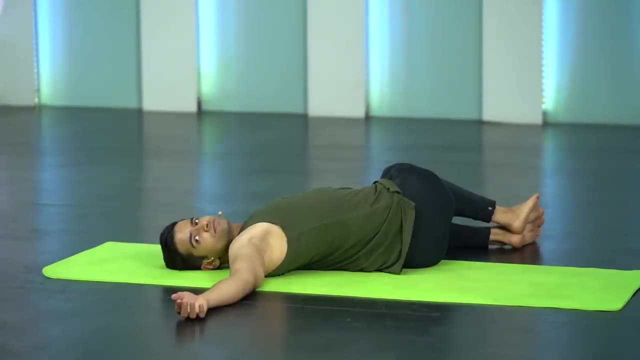 2,, 3,, 4, 5,. slowly bring your knees back to the center, exhale, taking it to the left, holding it there. 1, 2, 3. feel the changes happening to the lower back. 4, 5. gently come back. 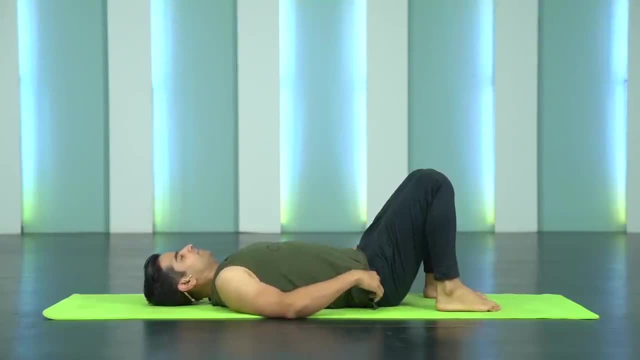 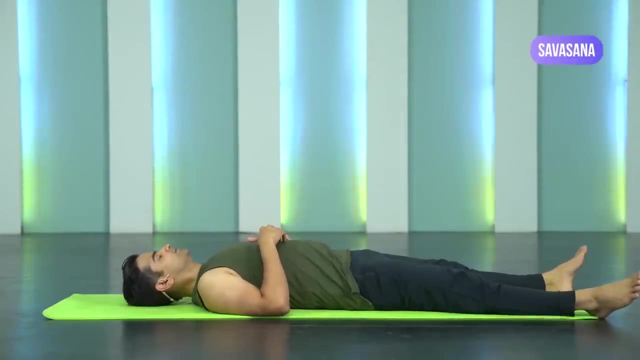 and relax your legs. now from there, just straighten your both the legs into savasana. make sure your both the legs are shoulder width apart. make sure your both the legs are shoulder width apart. turn the toes down palms by the side of your body slightly away. 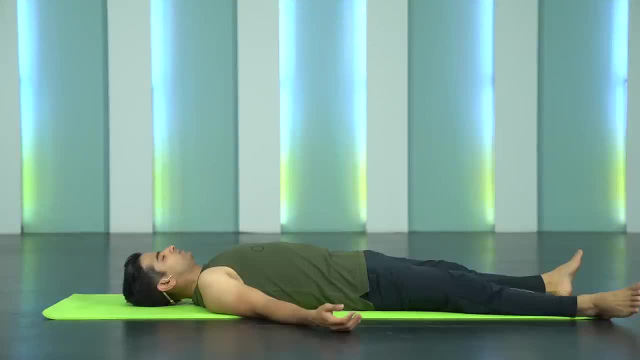 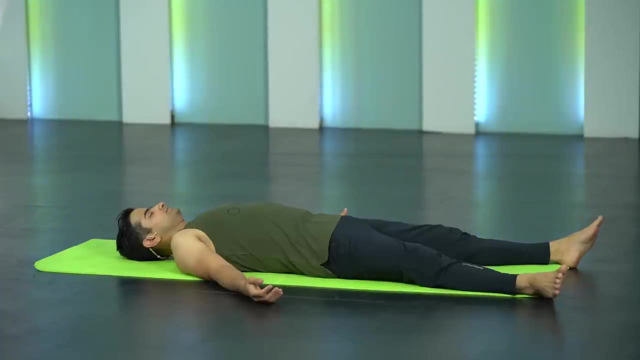 keep your eyes closed, lower back settled on the mat. let us just breathe in, breathe out. every time you are inhaling, feel the expansion of your belly. feel the expansion of your belly every time you are exhaling. feel the expansion of your belly every time you are exhaling. 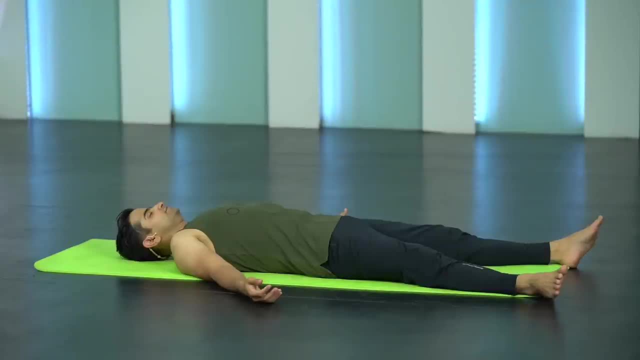 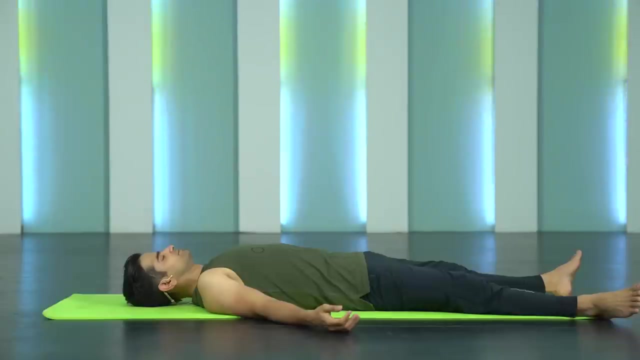 feel the expansion of your belly. keep inhaling and exhaling with a lot of awareness, with a lot of awareness breath. your body and mind are becoming relaxed. Your body and mind are completely relaxed. Start to become aware of your surroundings: sounds in your surroundings. 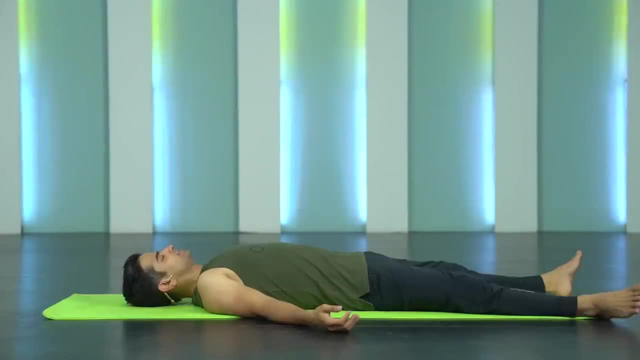 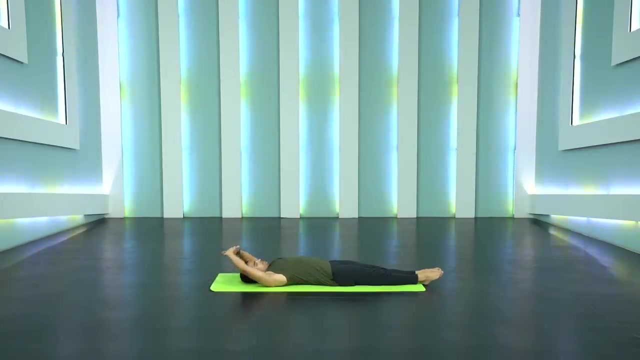 Slowly come back to the body consciousness. sensitize your toes, your palms, Bring your legs closer. let us stretch the hands behind, Toes pointed. Now loosen up your hands completely, fold your legs, taking a turn to the side. 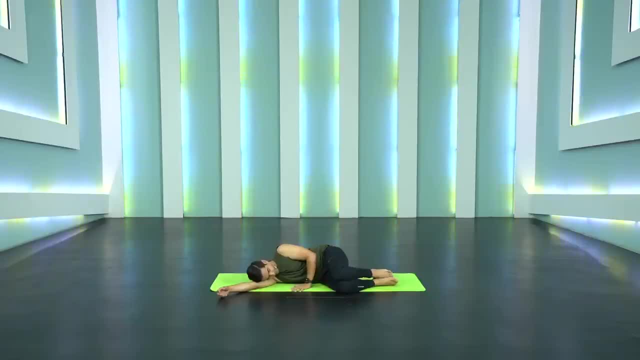 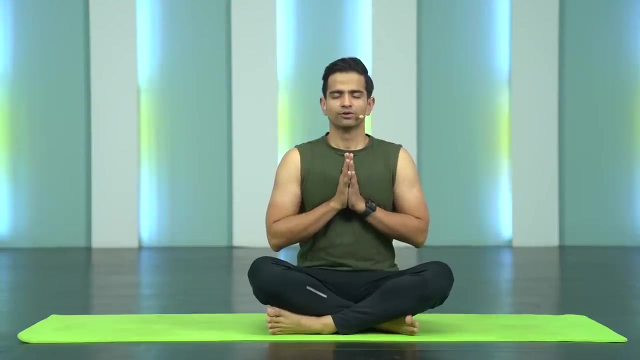 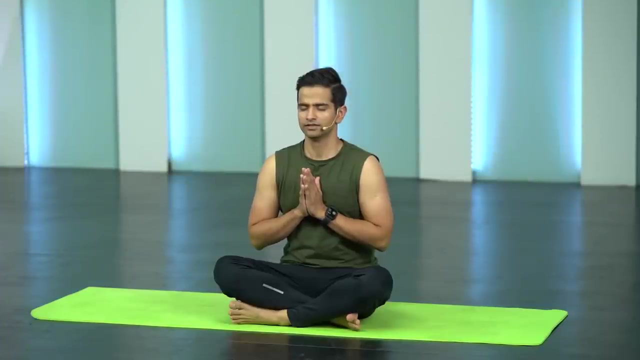 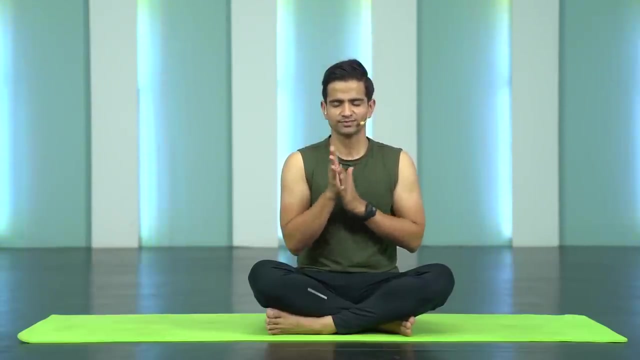 Give support to your head, Coming back and sitting in a comfortable position With your eyes closed back, straightened Palms together. in Namaste, We will settle down all the energies For today's practice. inhale. Let us start to rub your palms, creating a good amount of energies in your palms. 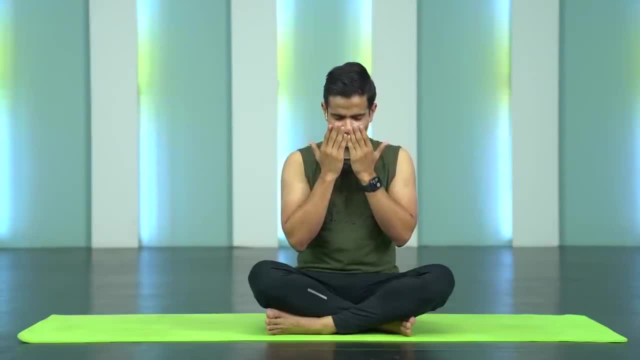 Bring your palms to your face Now, slowly look at your palms with a beautiful smile and a few blinks. All right, So this brings us to the end of our session. Today I shared one of the ideas that I follow to create triggers to follow my healthy habits. 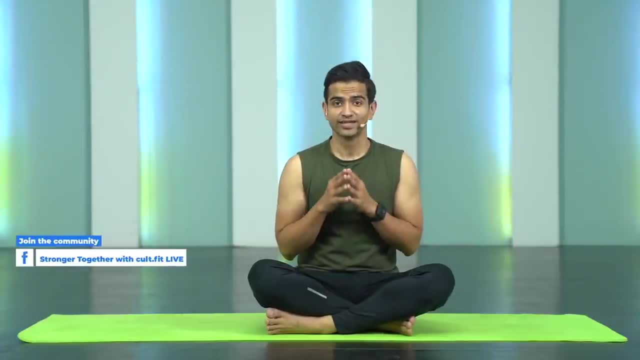 I am sure you also have a lot of ideas, So make sure you share those ideas on our Facebook community Stronger Together. I will be very happy to see them. I will see you in my next session. Until then, this is Naveen here signing off. Namaste.